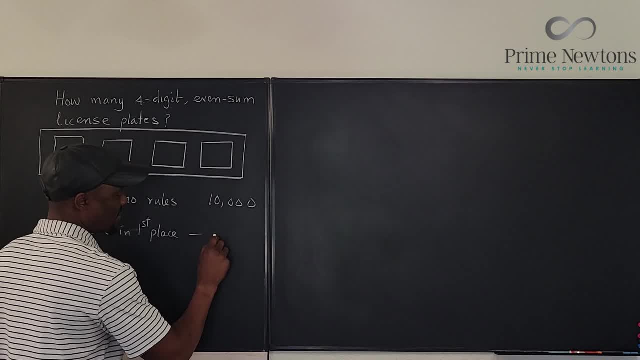 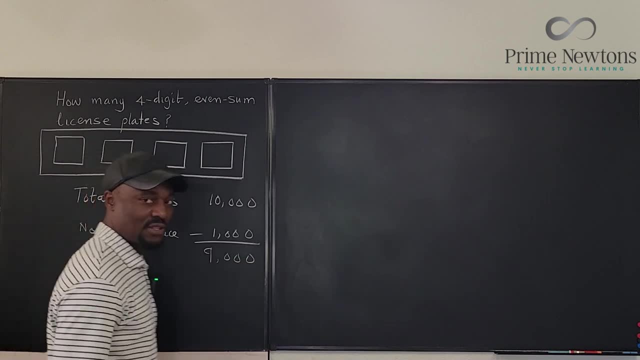 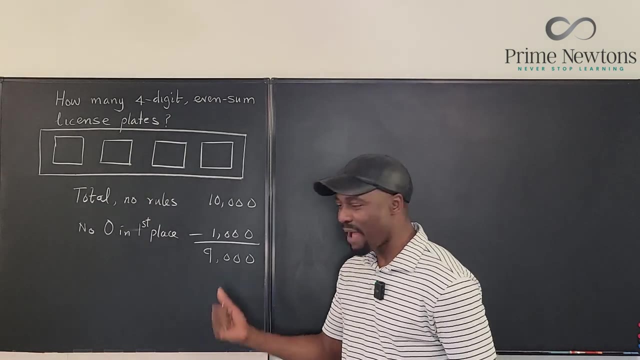 So now, with the restriction, no minus 1,000.. So now, what we have left is 9,000 license plates. Now I'm writing this as an accountant, Okay Now. so what happens to the remaining 9,000?? Any number you pick is either even or odd. 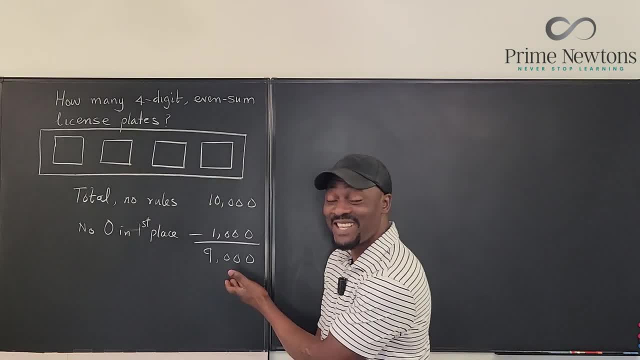 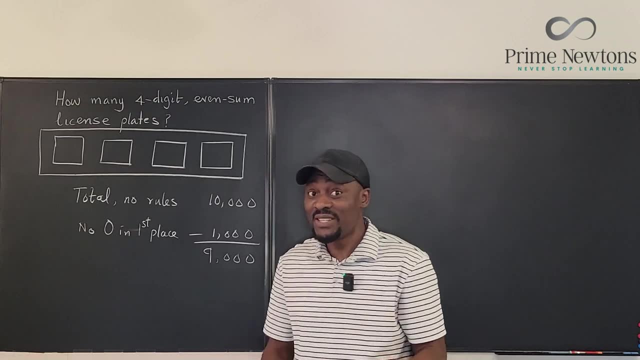 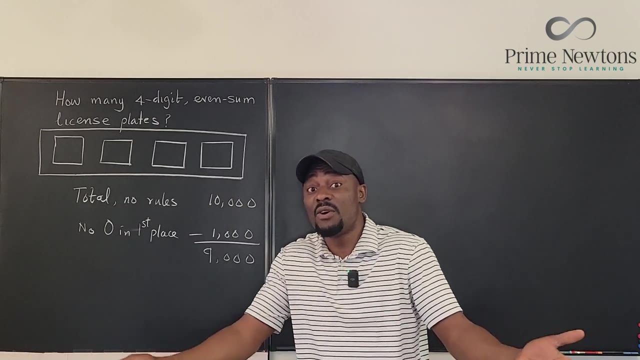 Remember that. So the remaining license plates. if the sum of the digits you take it, it is, either it is even or it is odd. There are no options. Every number you get when you add anything up is either even or odd, unless it's 0, where some people say we don't know if it's. 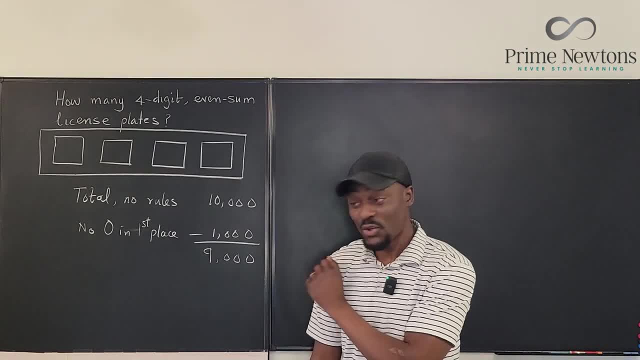 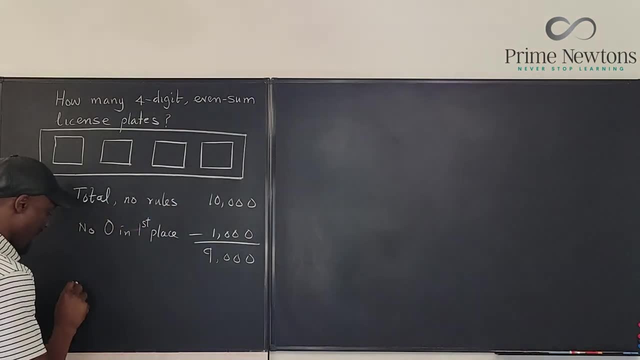 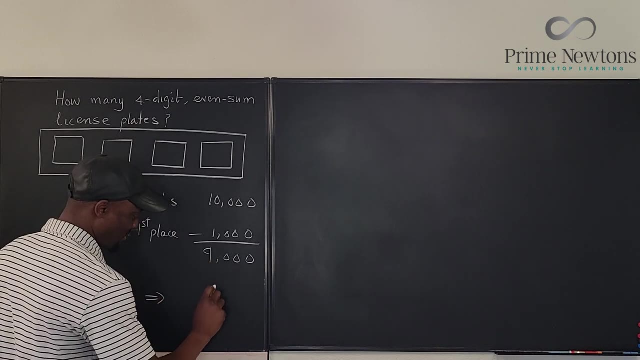 even or odd, But that's, That's it. So half of these plates will be even and half will be odd, And that's it. So we say half even implies we divide this by two. So half even, half odd. Okay, let's do this: Half odd. 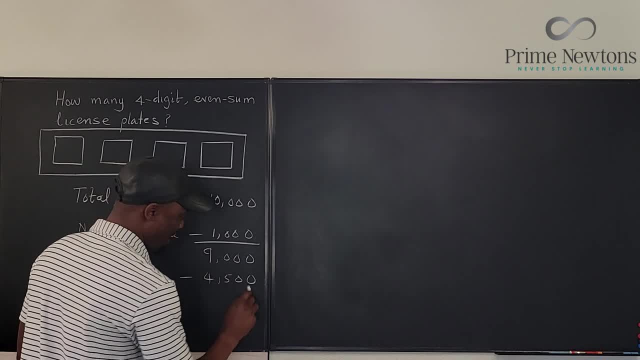 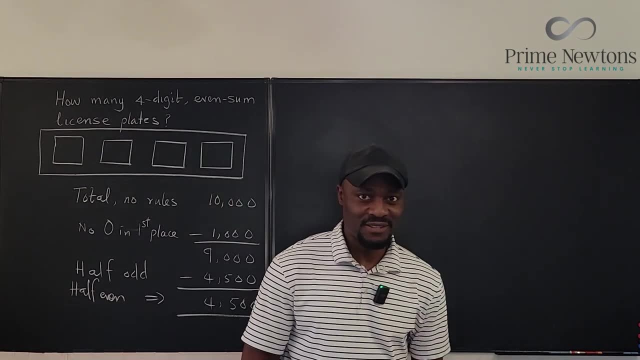 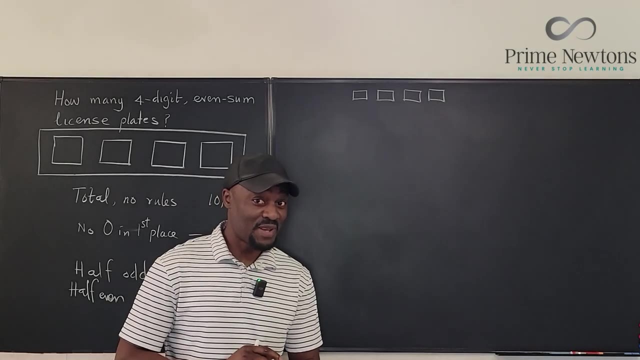 we subtract 4,500.. What is left will be 4,500.. That is the accountant's method of solving this. Now let's go to the mathematician's method of solving this. So this is how a mathematician will reason this out. I want to put numbers in this to form my license. 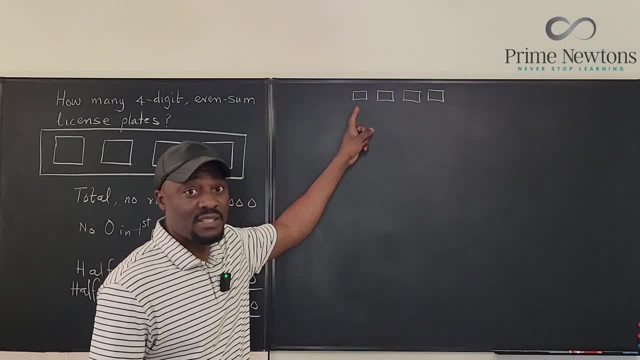 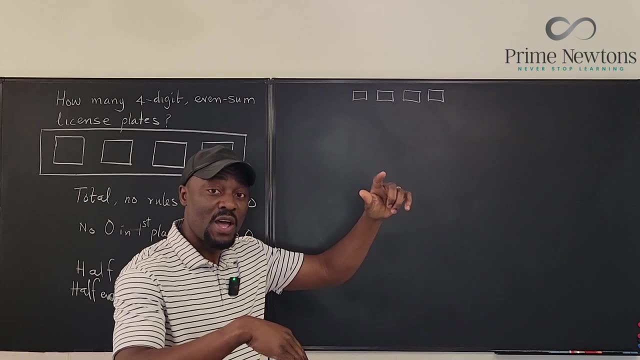 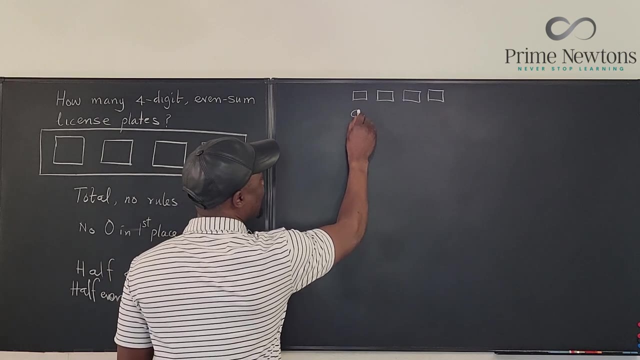 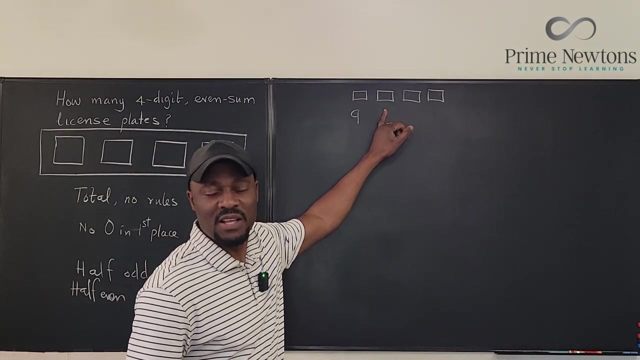 plate. What are the rules you gave me? You said the first digit cannot be zero. So of the list zero to nine, I have to drop zero. I only have nine numbers that I can plug in here, So I have nine. Now I'm going to go to the second digit. Nothing about the second digit really calls for. 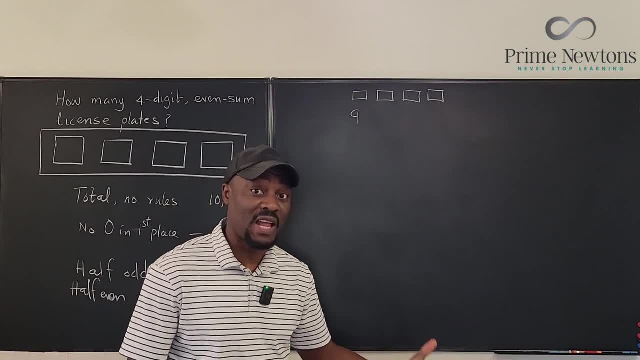 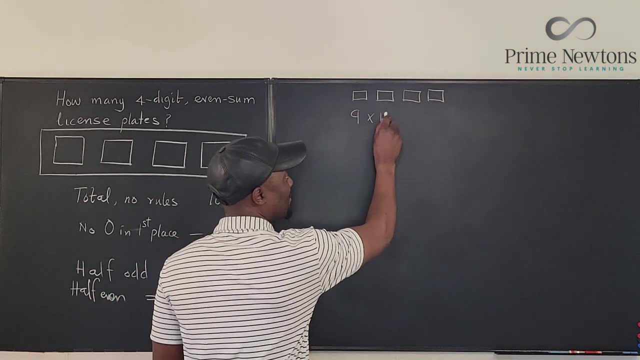 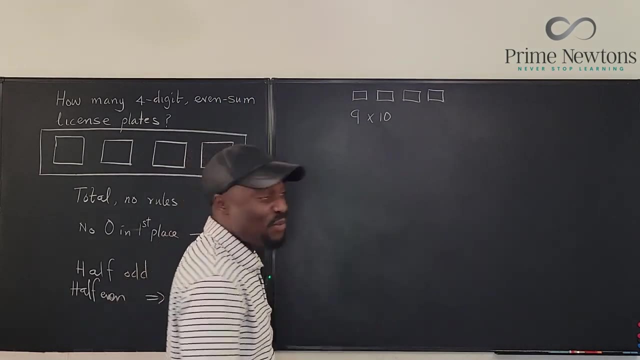 any attention, Anything can be there And because there is repetition allowed, whatever number I've used here, I can also use here And I can also use zero. So I have 10 options. The same thing here: I have 10 options, No restrictions. 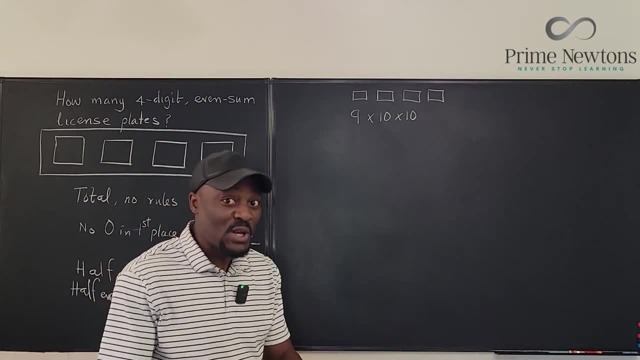 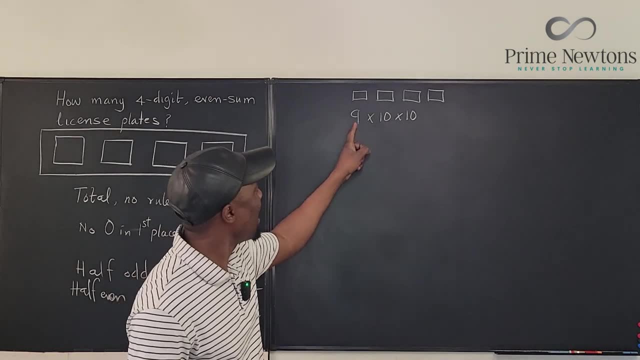 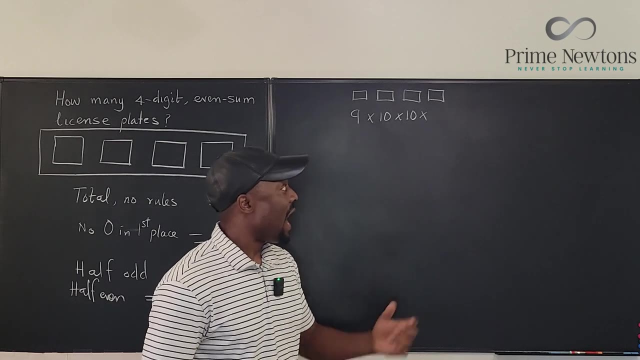 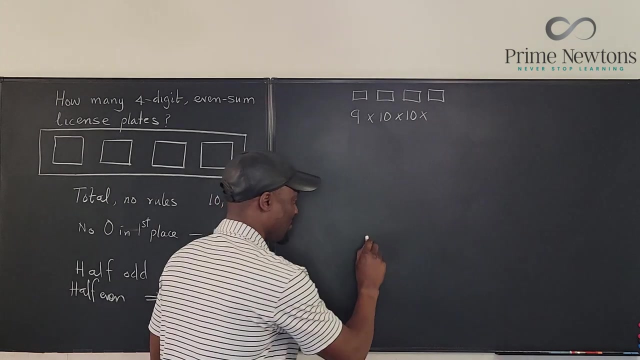 Now I have to slow down. I cannot say I have 10 options here, because if the number that I have right now- I have 900, right Now for the last position- I must ask myself: do I have 10 options? No, because if currently the numbers I have arranged together, let's say I: 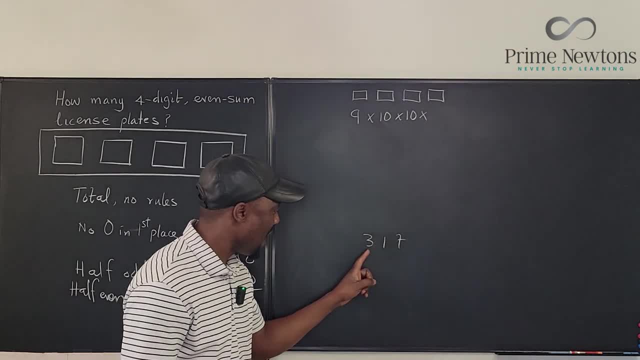 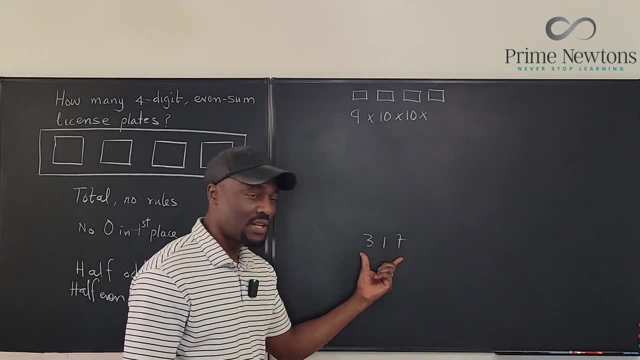 have three one. seven is the number I chose. I'm going to add: three plus one plus seven is going to give me 11, right, Is 11 an odd number? Yes, Well, I have to be careful what number I put. 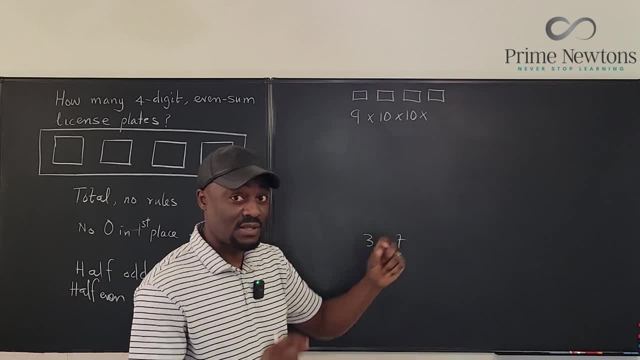 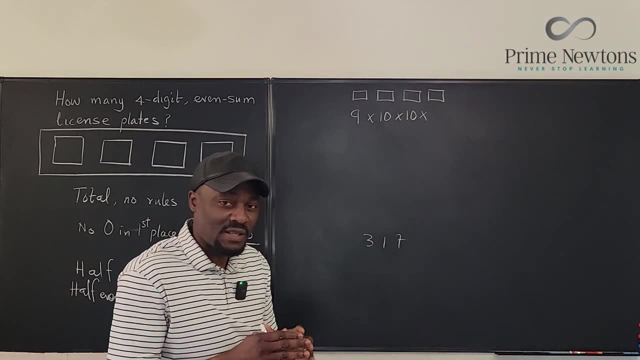 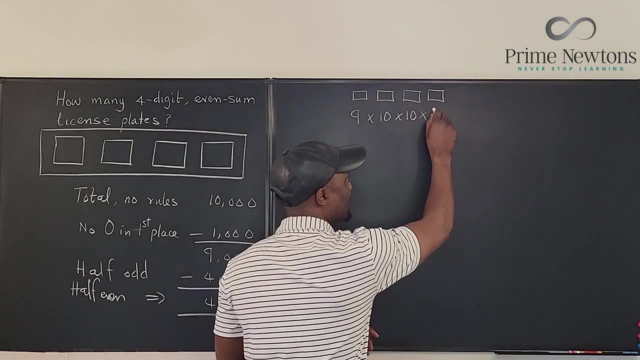 here I must put another odd number, because the sum of two odd numbers will be even. So I cannot put an even number here. I am restricted to just one: three, five, seven and nine. So I have five options in the last spot. Oh, what if it was even? 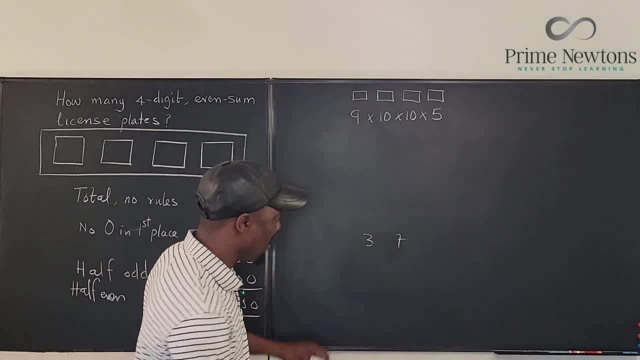 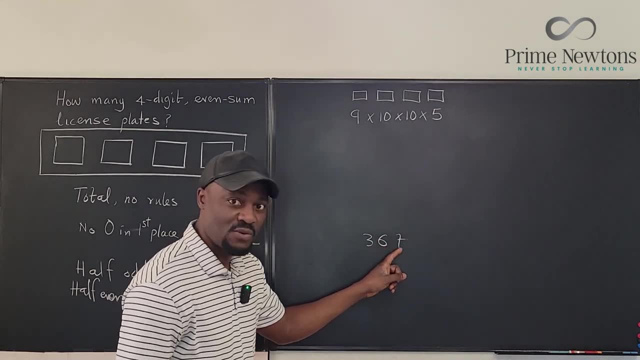 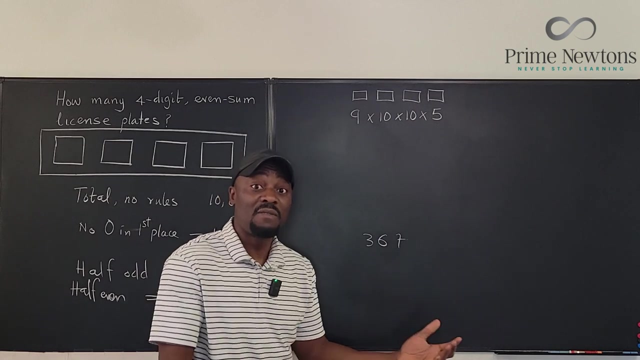 It's the same reasoning. Suppose that this was not one, it was say six. If I add up the digits, I'm going to get nine plus seven, which is 16.. It's an even number. So how many options would I have? if the first three are even, I will still have five options. I have to choose either zero. 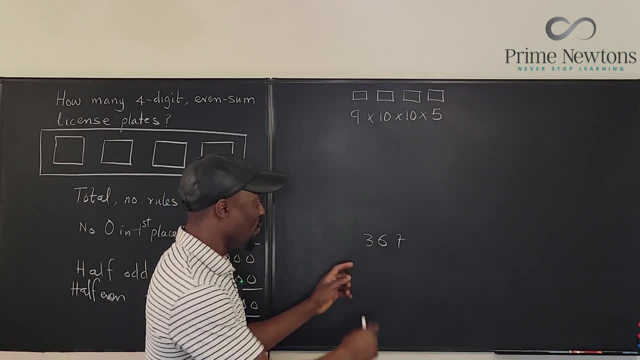 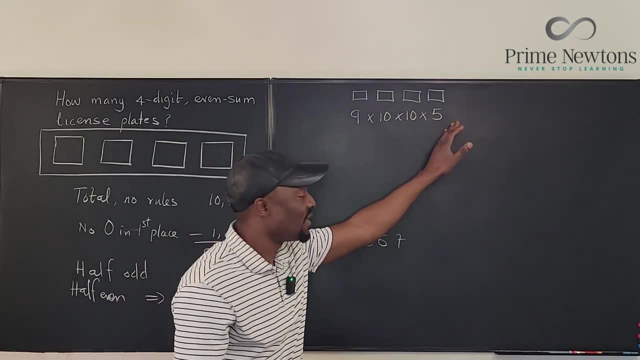 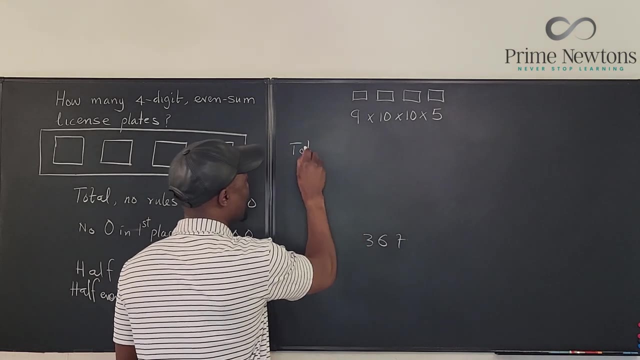 two, four, six or eight, So I still have five options. So whether what I have here is even or what I have here is the sum is odd. the last option I have will have to be restricted to five, So our total is going to be nine times. 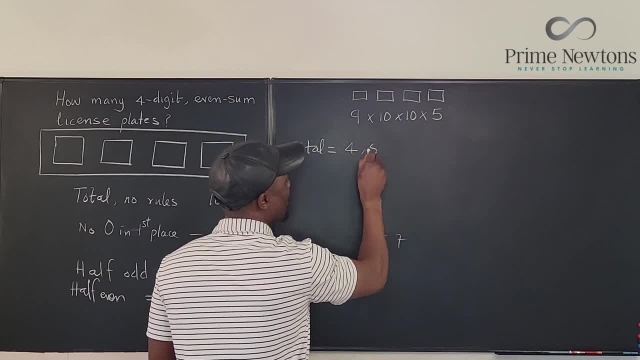 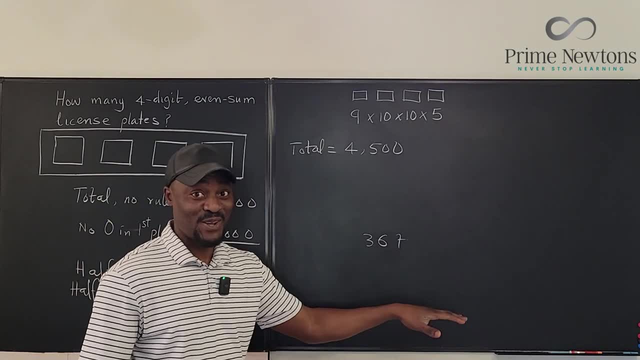 10 times 10 times five, which is 4,500. by that reasoning, I did not want to write, because there's another way you can do that. Now, what's another way you can go about this? And this one is what. 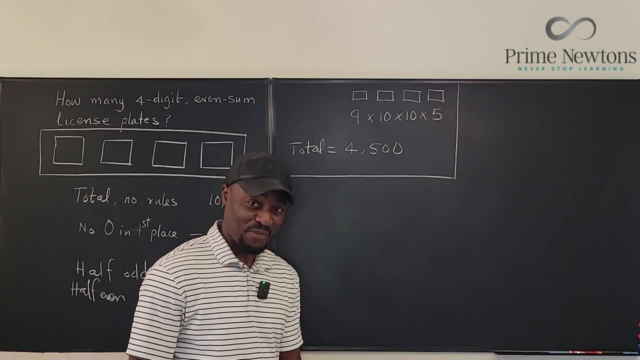 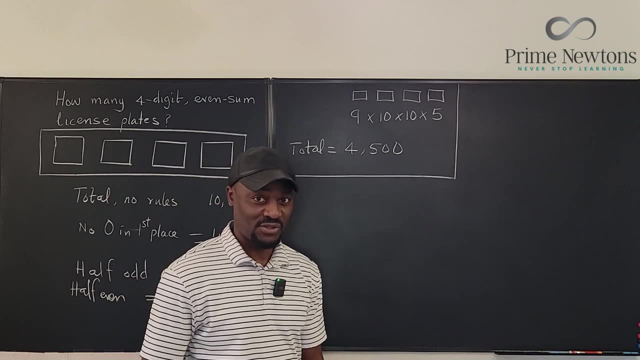 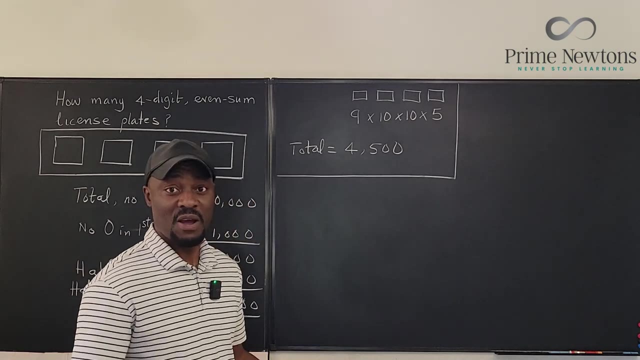 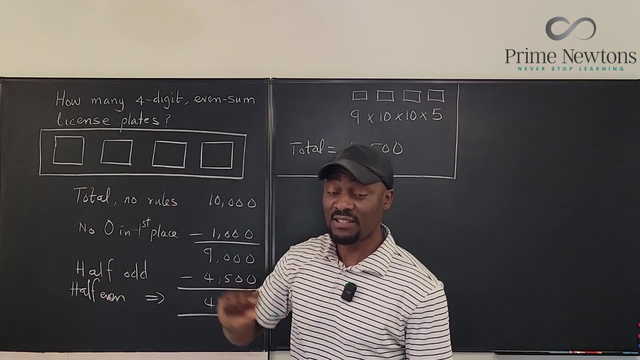 I think the teacher is looking for, Because you're not expected to know this combinatorics method. You're expected to use arithmetic progression or what you call arithmetic sequence. Okay, so we're going to have a sequence of numbers And let's look at the question again. What is the very first number? license plate with 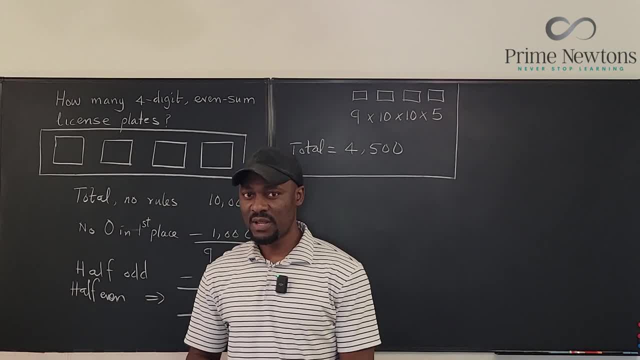 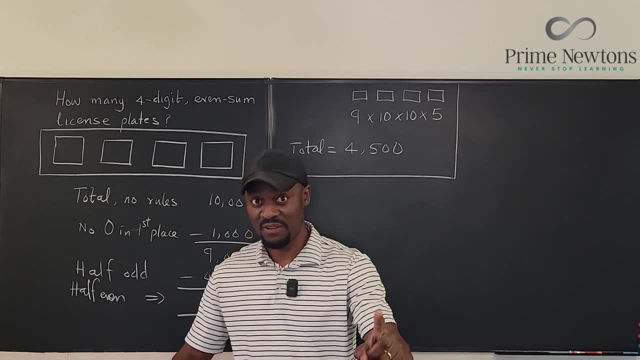 the smallest sum that you can accept in the sequence, Can you accept? Okay, so since we said the first digit cannot be zero, the first digit must be one for the smallest one. So it's going to be one: zero, zero, zero, no. 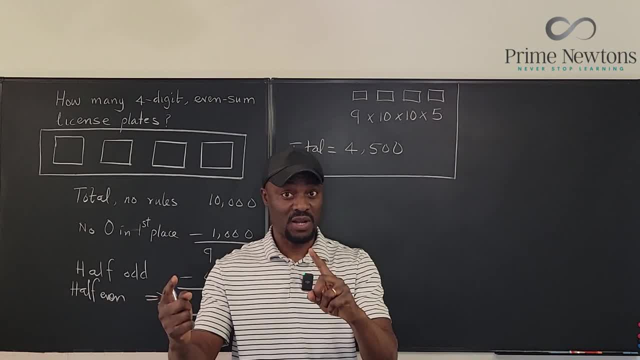 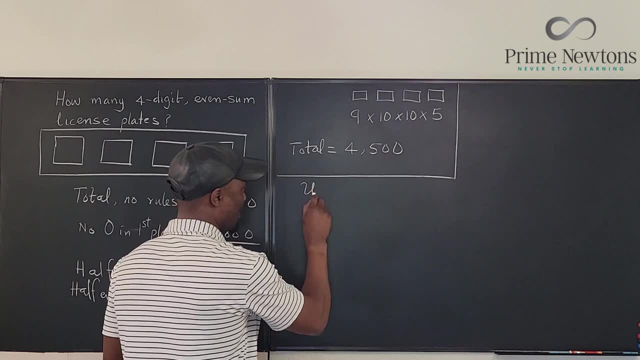 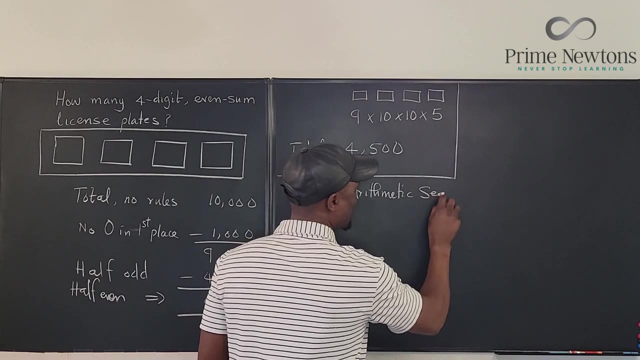 because when you add those up you're going to get an odd number. it's one. So the smallest license plate sum is going to be two, because the first license plate. so, using arithmetic sequence, So that's what we're going to be using. So we're going to say: 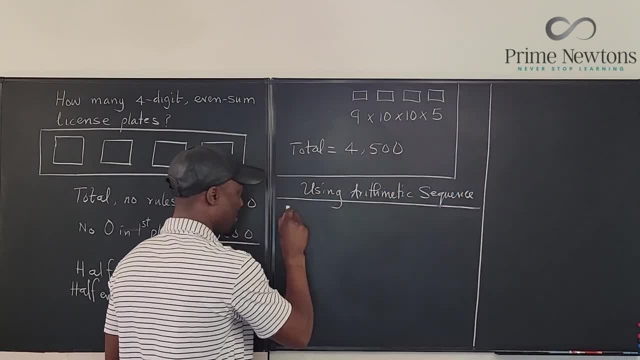 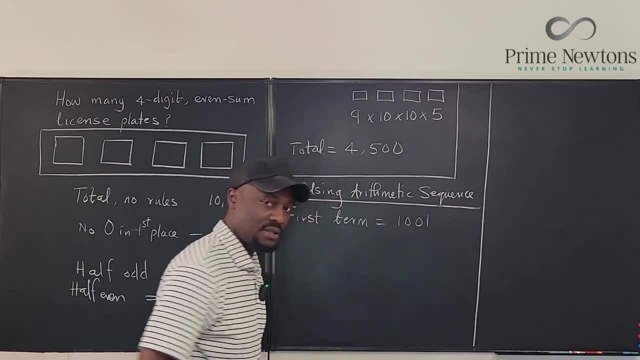 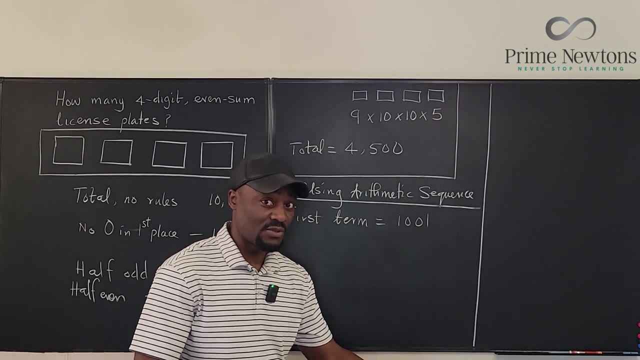 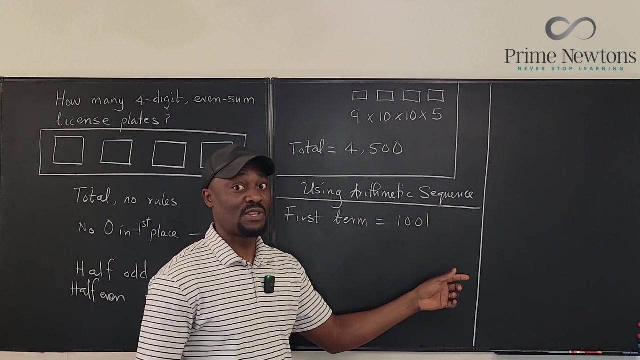 hey, let's stop this off. The first term is 1001.. This is an acceptable license plate. 1002 is not acceptable. 1003 is acceptable because this one will give us a sum of two, which is even. 1002 will give us a sum of three, which is not even. So it looks like the next. 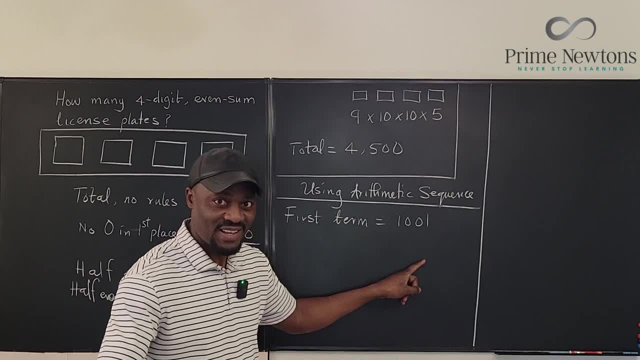 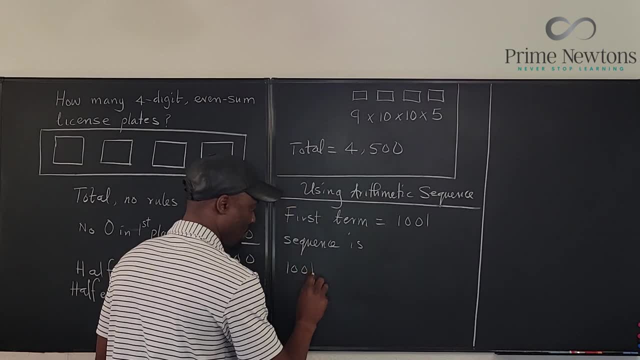 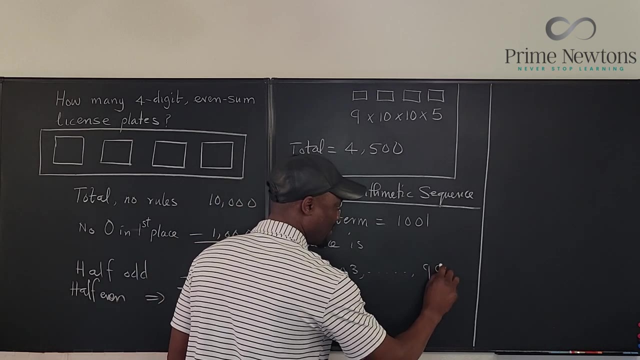 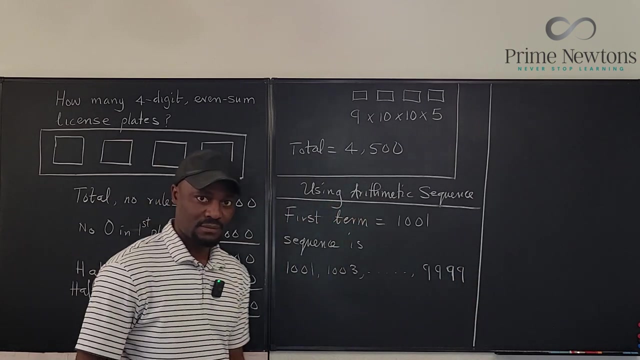 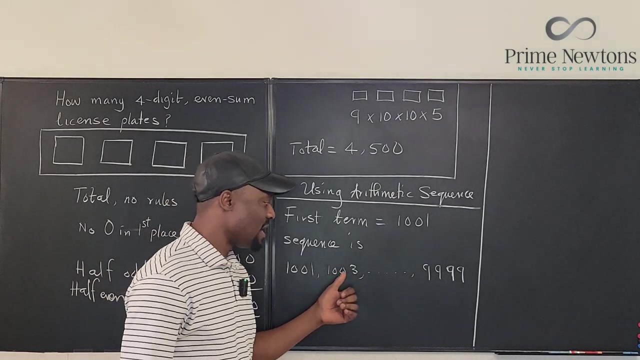 number is going to be 1003.. Okay, so sequence is 1001, 1003, tap, tap, tap. you keep going until you get to 9999.. That's it. The only question you want to ask yourself is how many terms are in a sequence? 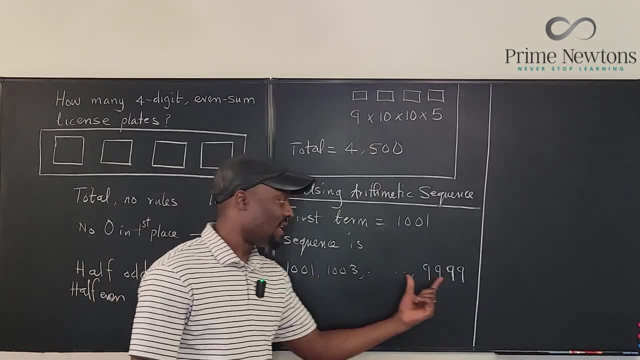 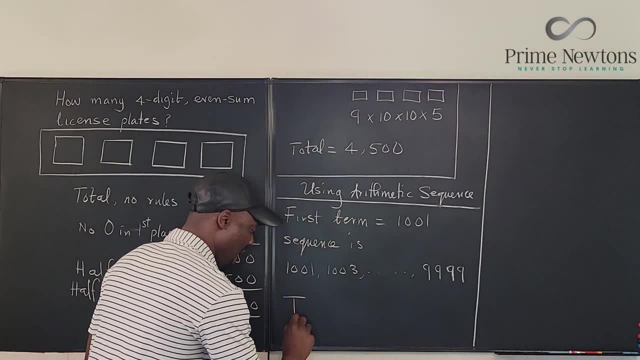 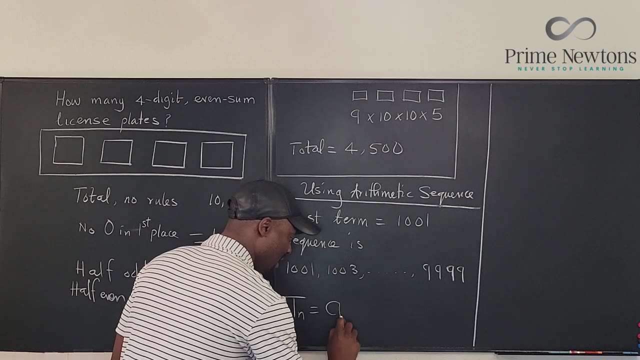 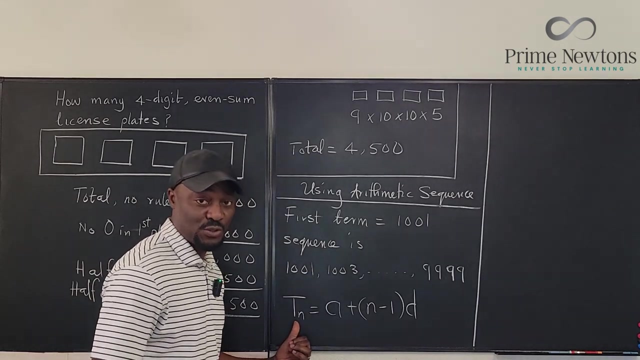 sequence where the first term is 1001 and the last term is 9999.. We know that term n for an arithmetic sequence or arithmetic progression is equal to a plus n minus 1 multiplied by d, where the term we're referring to- whichever term this is, we just pick it- is the first. 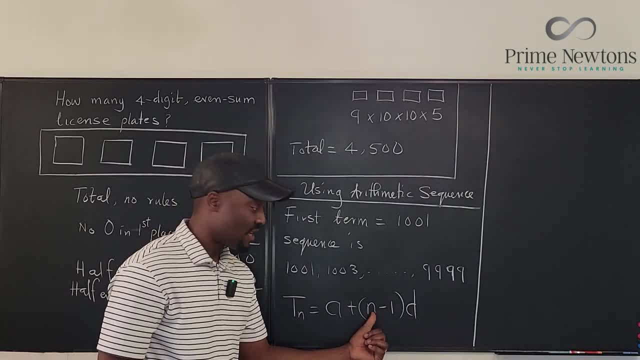 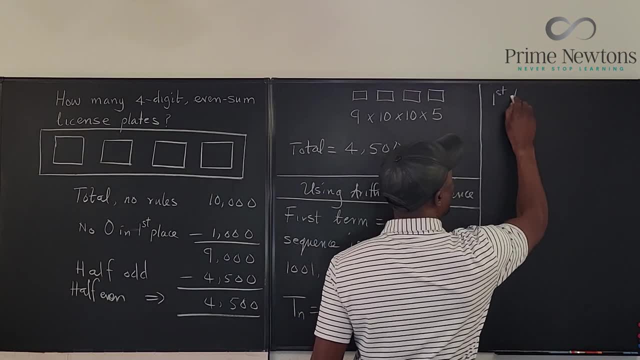 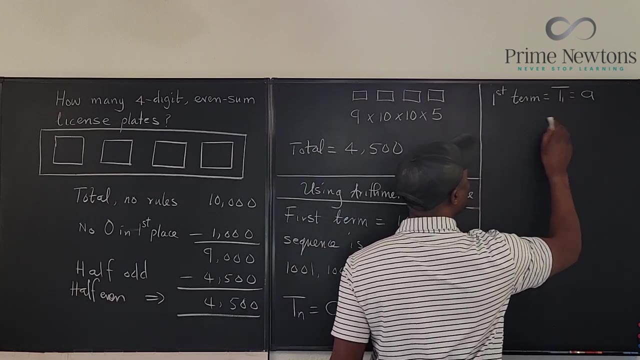 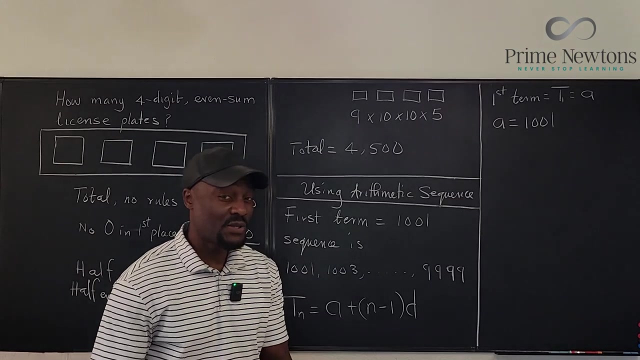 term multiplied by the number of terms minus 1 multiplied by the common difference, We know that the first term is what we call t. I'll call it t1, it's also a and our a in this case will be 1001.. So if you're in high school, this is what you're more likely going. 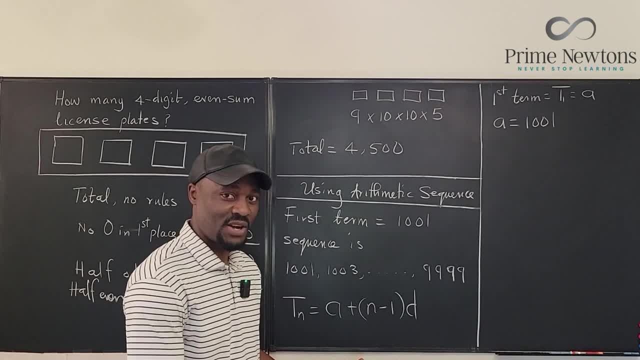 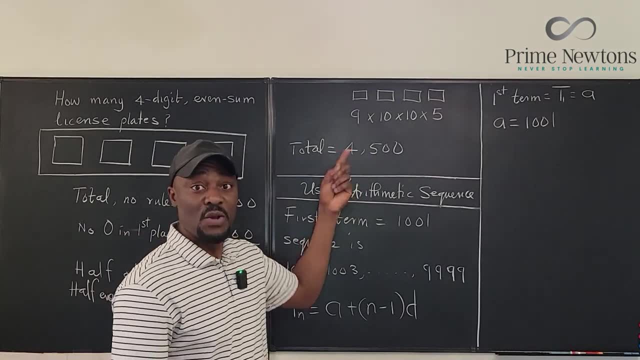 to present, okay. Okay, If you're in high school, this is what you're more likely going to present. okay, If you have done combinatorics or in further mathematics or advanced mathematics or number theory, this is what you might do. And if you're just someone who uses basic logic, 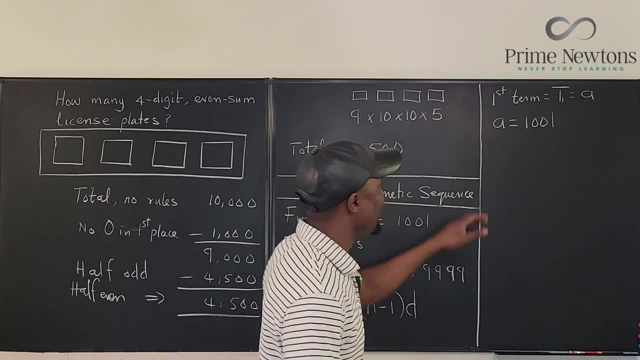 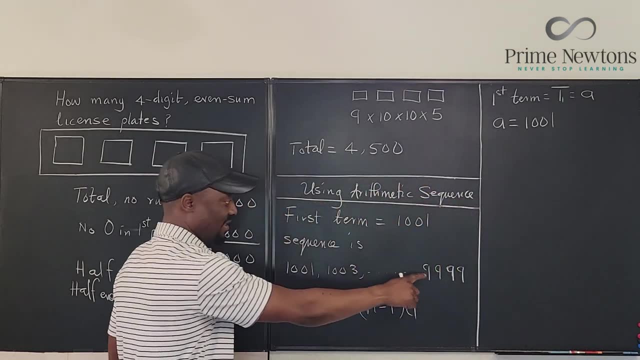 this is what you might do. or, if you're an accountant, Okay, In this case we have it- a is 1001.. What else do we need? We know that, So we're going to take this term, okay, We. 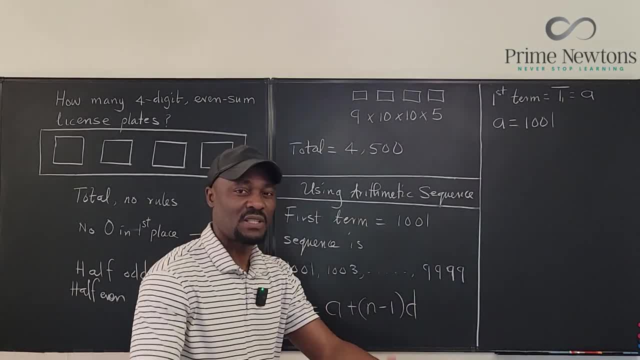 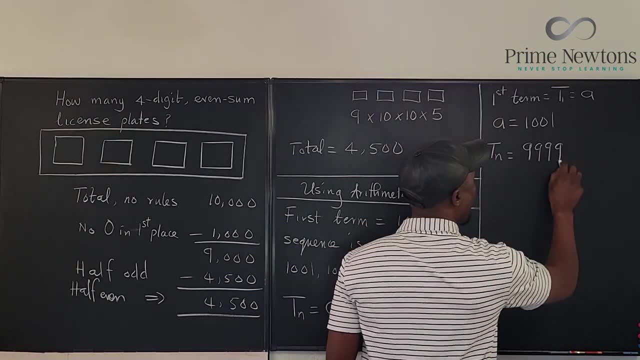 don't know what the term is, but it is the nth term, which is the last term, So we're going to take this term, so we call it tn. it's going to be 9999.. We just don't know what this n is, which is the number of terms, which is the number of license plates. we're 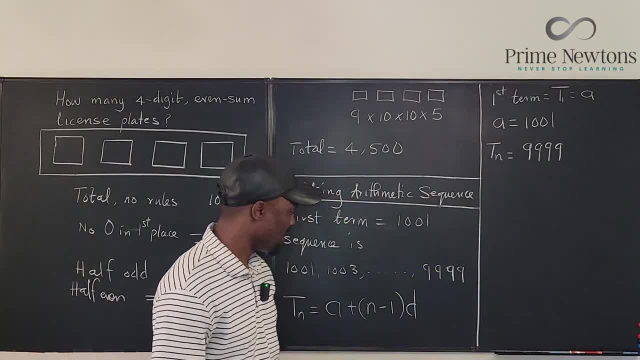 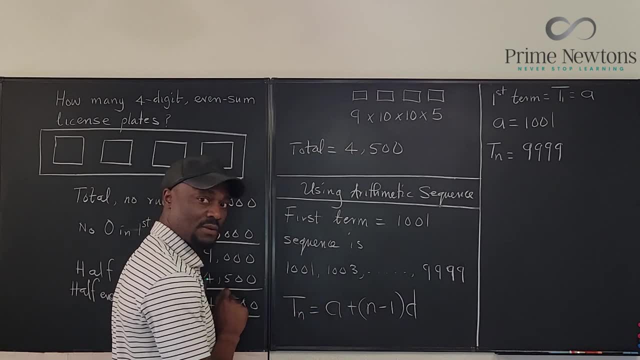 actually looking for. So tn is 9999.. What else do we not know? The common difference. What is the difference between this number and this number? What did we do to this? We added 2.. So every time you're going to be adding 2, d is equal to 2.. So we're going. 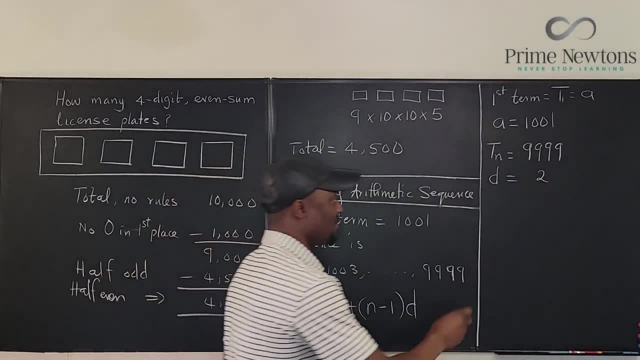 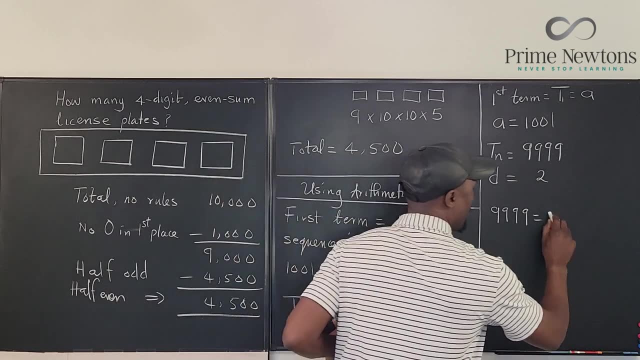 to go back and use this formula and find what n is. So tn is 9999.. What is the difference? Well, here we go. We have. 99999 is equal to the first term, 1001, n minus 1 times 2 plus. 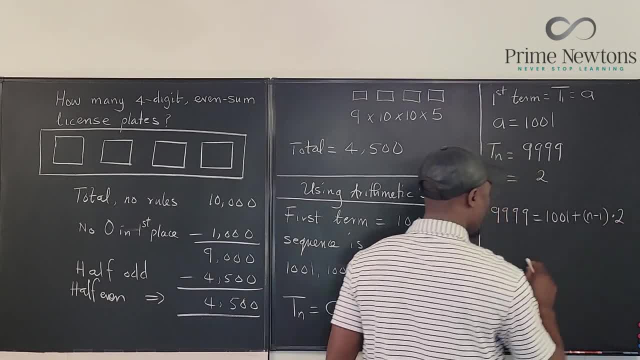 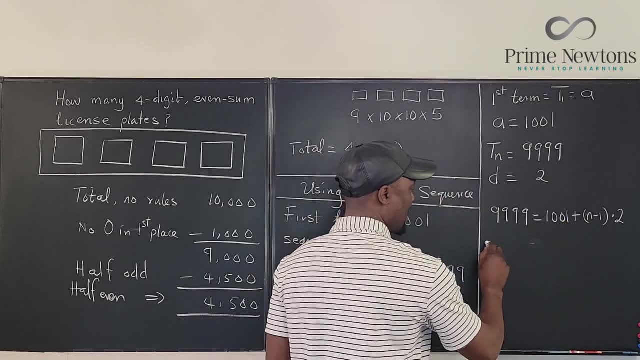 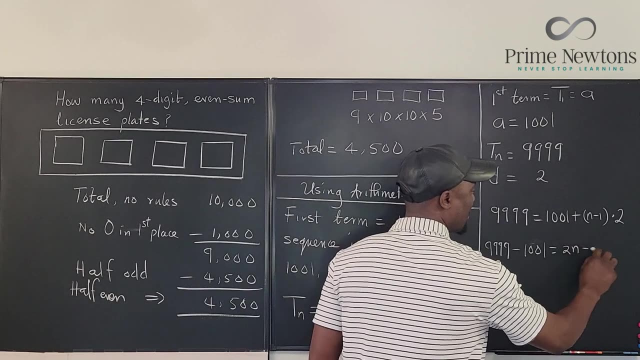 n minus 1 times 2.. This is going to be equal to: we can actually move this over here and say this is going to be: 99999 minus 1001 equals 99999.. Okay, Plus 2n minus 2.. Okay, I distributed this. So if we do this subtraction, we're going. 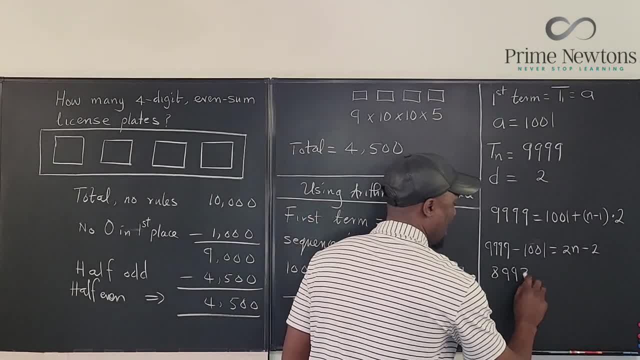 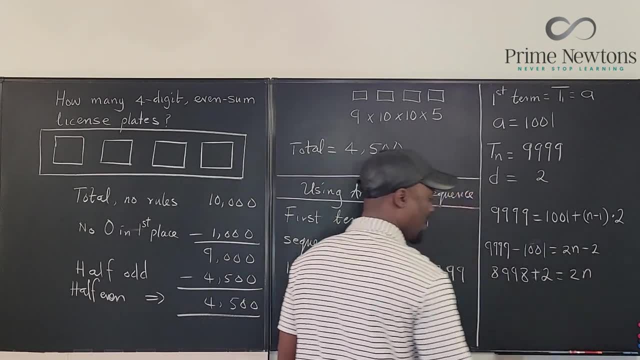 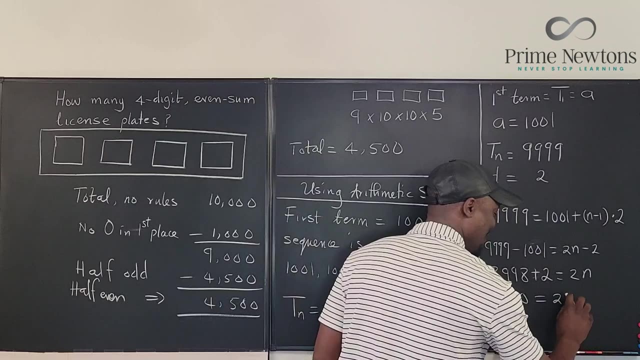 to get 8998 equals, and we can move this 2 here. so we add 2, plus 2 equals 2n. Whoa, If we add 2 to this, we get 9000 equals 2n, So that our n is 4500.